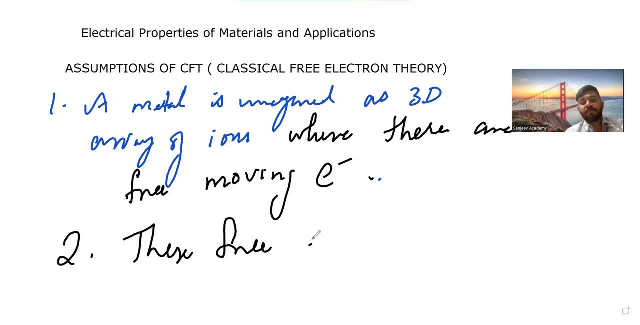 These free-moving electrons cause conduction. These free-moving electrons, these free electrons cause conduction. Or why metals are considered good conductors of electricity? Because there are electrons which moves. So already we know these things. Assumption of classical free electron theory. 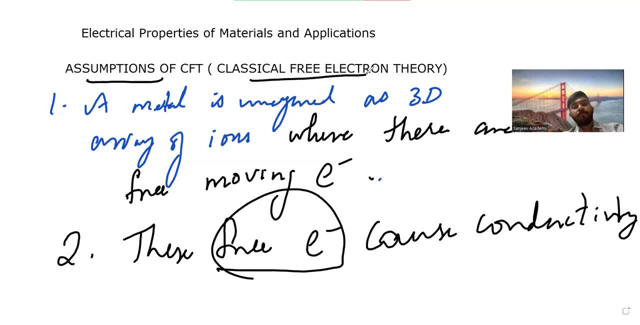 So this is nothing new, But again it has got some Effects That will try to prove that this classical free electron theory is wrong also. Okay, So that is in the next part. So this is our second point. 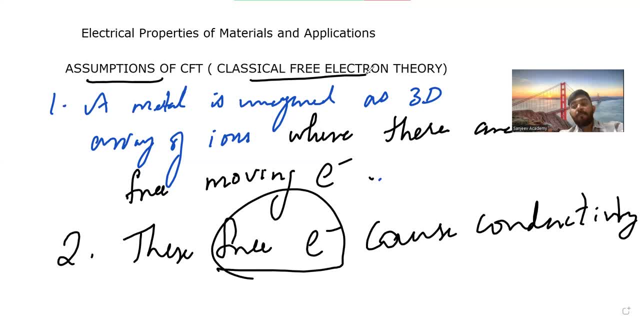 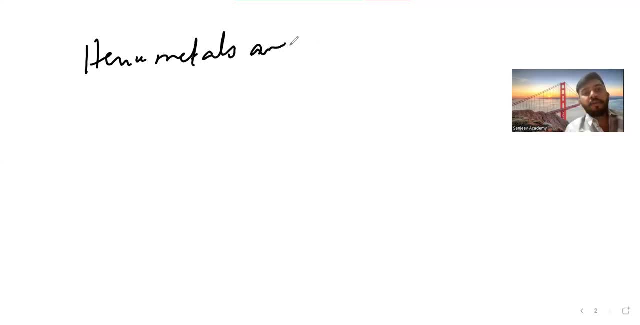 So the free electrons causes conductivity. Hence metals are Hence. Hence metals are good conductors of electricity. That is due to this only Clear Yes, Then, before moving to the third point, I just wanted to know: 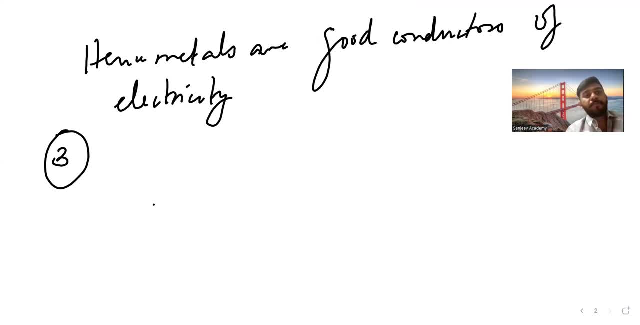 Yes, There is a term called drift velocity, Drift velocity, There is a term called drift velocity, velocity. So drift velocity, because the next point is related to drift velocity. So, before knowing that, we should know what is drift velocity, right? So drift velocity is nothing. 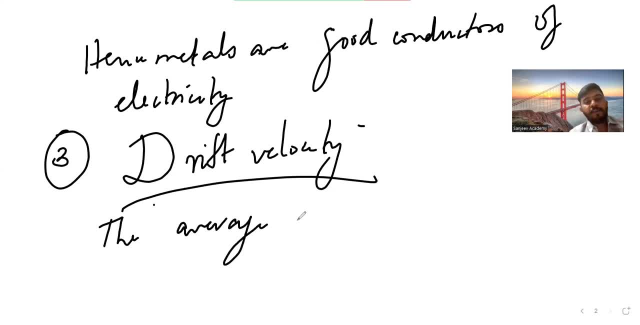 but the average velocity. I will write down in words the average velocity, correct, of occupied. the average velocity occupied by the electrons, by the electrons in the steady state. in the steady state in applied electric field, in applied electric field. The average 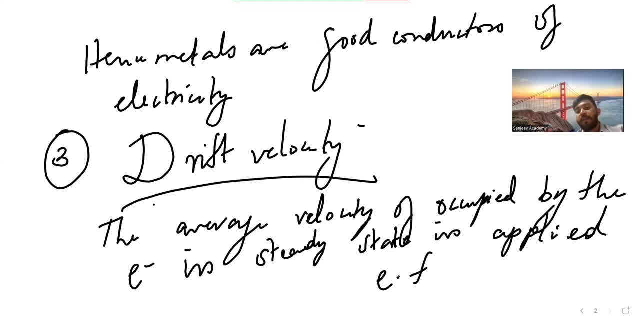 velocity occupied by the electrons in the steady state in applied electric field. This EF is nothing but My electric field Electric field. This is called drift velocity, See, but I have written here the average velocity of occupied. So again in examination, if you are writing off, 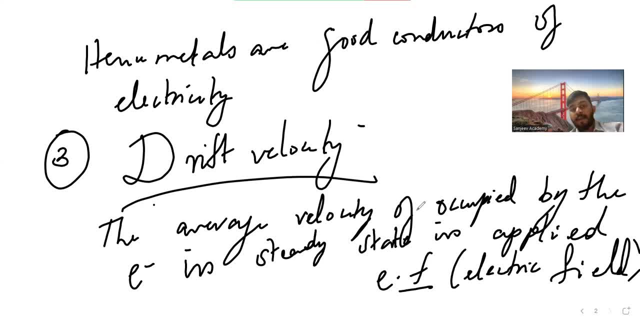 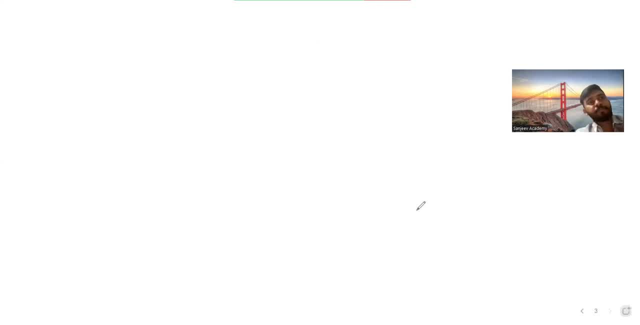 or some grammatical error. kindly do not scratch it, Kindly write it as it is. Now coming to my third point. so this is drift velocity. So third point is nothing but the electric current. What is the cause of this electric current? 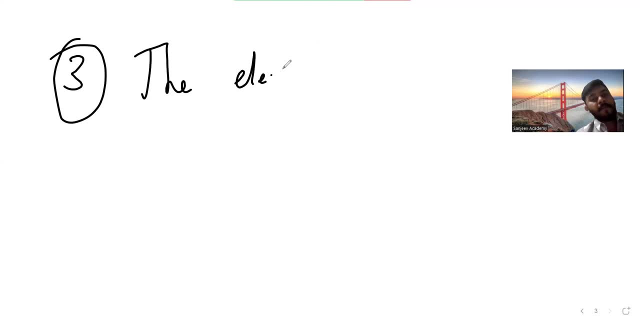 Correct The electric current. the electric current in a metal- correct in a metal- is caused due to drift velocity. Drift velocity in the sense, so the electric current is. how can this drift velocity suffer? How can this drift velocity cameratically, which we have written up over here. How can this drift velocity cumulative permitir, insert that condition into terms? Here you can write down towards closed pattern. So esquaring is the final part of the. what I mean by this left column. the initial element here is the half. square volume principle, and what you can write here is the cap, Because, using the cap as a constant, what you are writing out- Okay, so the electric current, all of these values- there will be the first two columns which will be measured at this behavior to Прothemator or: 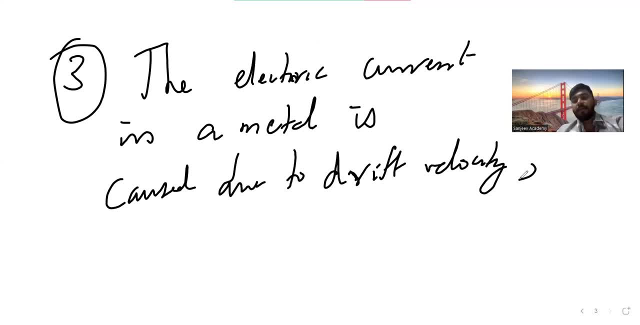 Metal is caused due to drift velocity, which means the electrons. I will write in different color. the electrons travel- this is very important- travel in opposite direction to that of electric field. Okay, so that is my third point. So I think you are clear with the three points. in electric field, 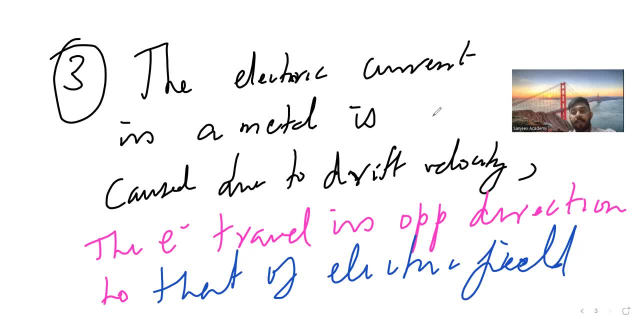 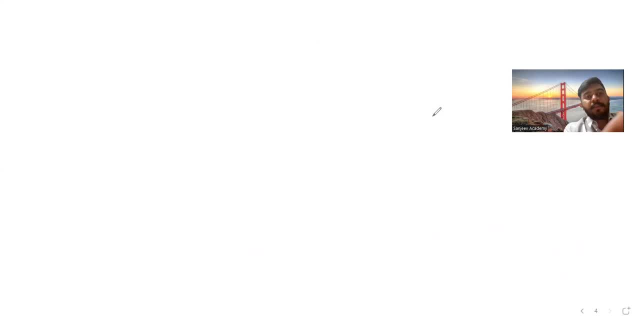 CFT: classical free electron theory. So the next topic is the next thing is thermal velocity. Thermal velocity- see, let's take this electron is here, right? this is in my electron Random. once it goes here, once it goes here. 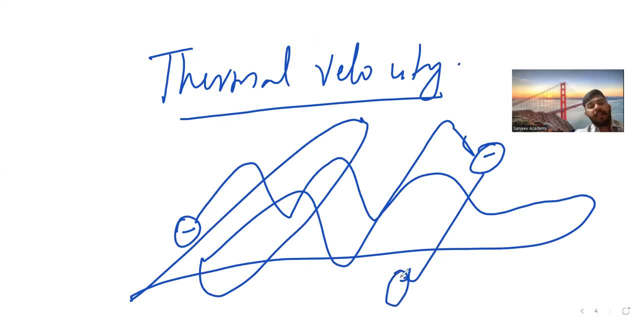 So basically, an electron is here. Sometimes it will be here The random, correct? This is basically random motion of electron, So that we have to keep in mind. So what is thermal velocity? I will write it down in words, correct? 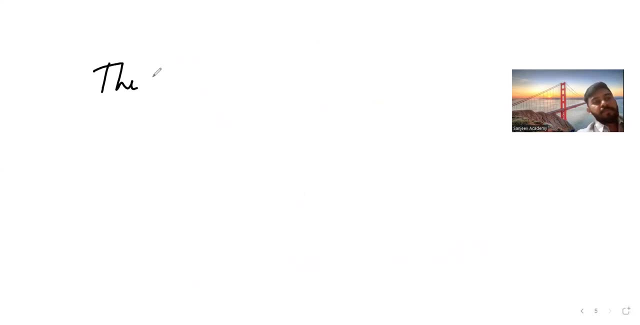 The velocity of electrons. The velocity of electrons in random motion Due to Due to Thermal Agitation Is called Velocity. Correct, For example, agitation. in a sense It's a different word. see, We also get agitated, the angriness correct. 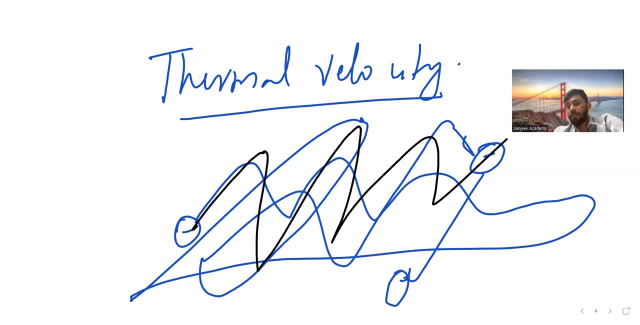 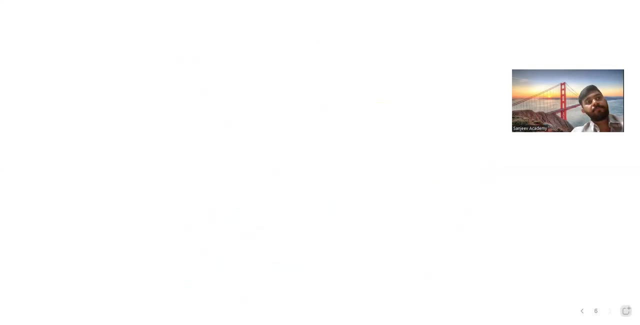 So we will do things which are out of control. that same thing also electron thing, but it moves in a zigzag manner or whatever manner. so this in a term is called thermal velocity. that's all. the next thing is: mean free path. mean free path, correct. so mean free path is a very simple thing. i'll write down in words so you'll understand. 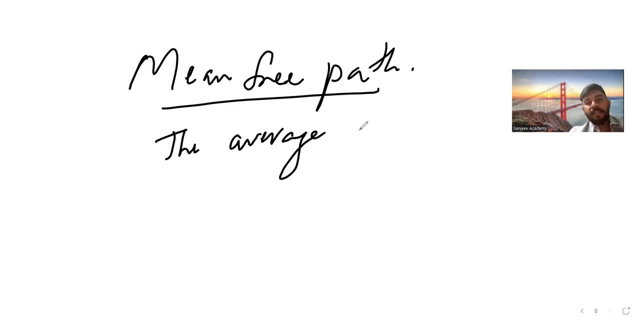 the average, the average distance, the average distance traveled by the electrons correct between any two successive collisions, successive collisions with the lattice ions, with the ions. this is called the mean free path- the average distance traveled by the electron between any two successive collisions with the ions, ions in the sense, other lattice ions before. 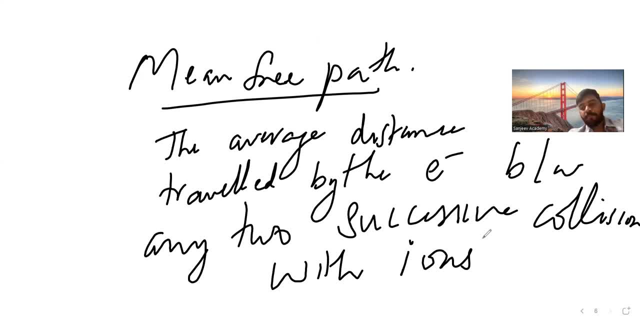 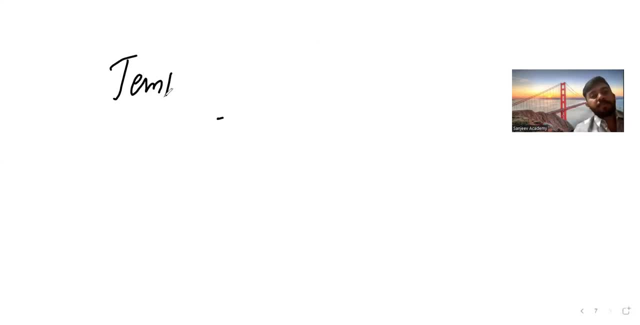 collision. next thing is: so this is a kind of theoretical thing. the next one is temperature, temperature, temperature temperature atiques, elements, elements on. on. what was this and what this mean? was earth taken from Democrats? when use energy, energy or energy is during. on, this is the rule. okay, so i'll tell you what is this method, sense, rule. i'll write down now. 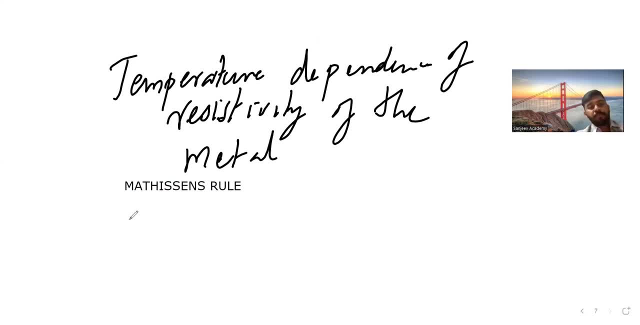 write it down. yeah, rho resistivity is equal to rho naught plus rho of p. this rho, this term, this is called. let me, i think you can able to see this rho. this is called by resistivity, correct? this rho of t, this rho of t is nothing but temperature dependence on the resistivity. 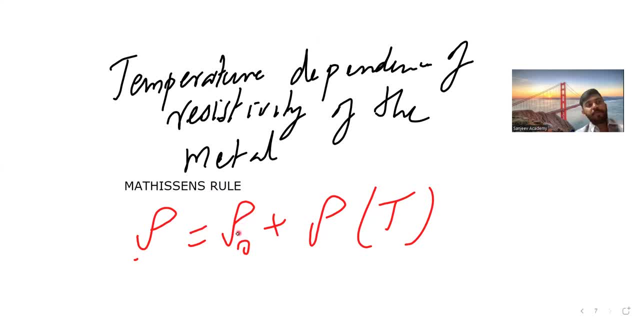 and this rho naught. what is the rho naught? this is called the residual resistivity. i'll write it down in words so you'll understand better: rho naught residual d-u-a-l dual residual resistivity. so this is my temperature, temperature dependence on resistivity and what is my rho. 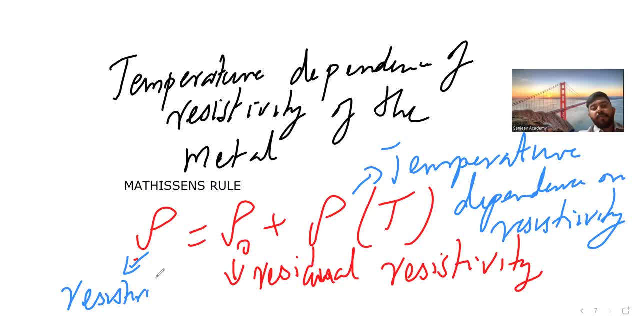 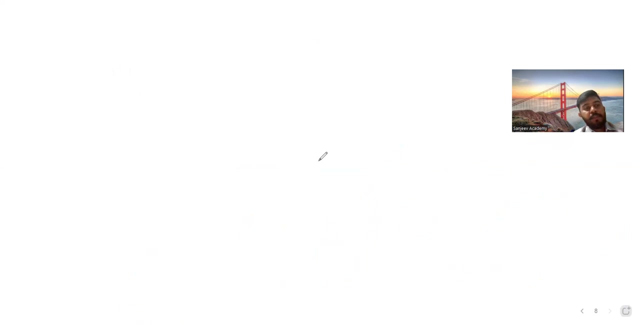 rho, resistivity of the given material, of the given material. okay, so this, this method sense rule is very, very important, okay, and we have to draw a graph of the same. so the graph also, these draw it. let me take this find, this will be my resistivity, this will be my temperature, which is in kelvin. so dependence of 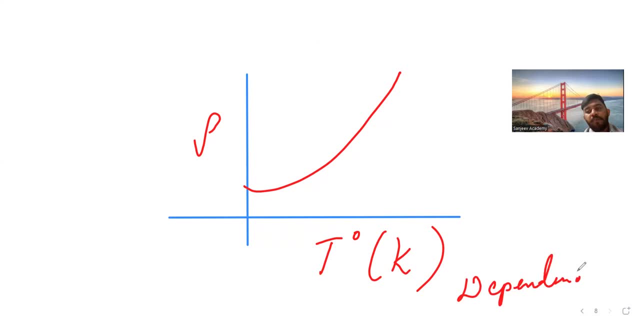 dependence of temperature- correct or raw- on temperature, on temperature. so this is how it is okay. and then you should ask me see the mathisans rule: basically, what raw is equal to raw? not plus raw of t? so what is this raw not? correct? this raw not is nothing. 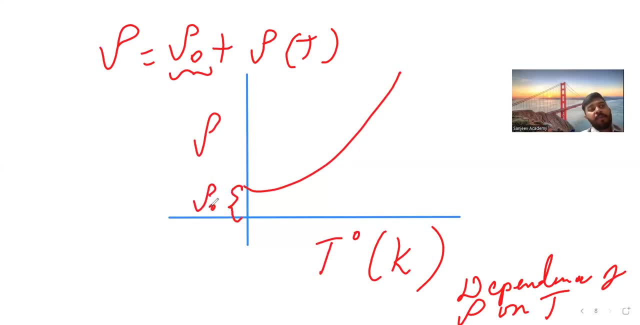 but this point, this point is the minimum raw, not clear. yes, this is called the residual resistivity. residual residual in the sense whatever resistivity is left out, that's it, residual resistivity. so so in our class 12th we have learned about residual magnetism. so there is a thing about 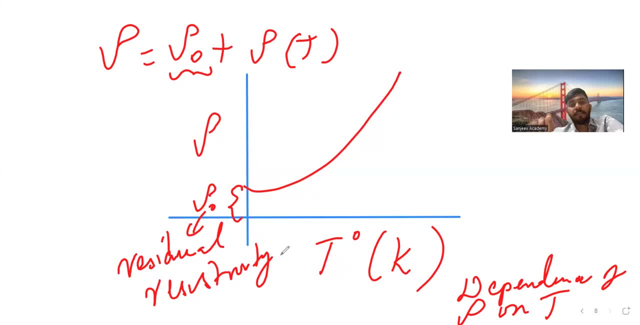 that magnet, which the magnetism property, the magnetic property which is left. even though if you remove the magnet, uh magnetism, from the material, but still the amount of magnetic property left, correct, that residual is nothing. so similarly for resistance. also, if you try to remove the complete resistance of that particular material, but still there will be a small amount of. 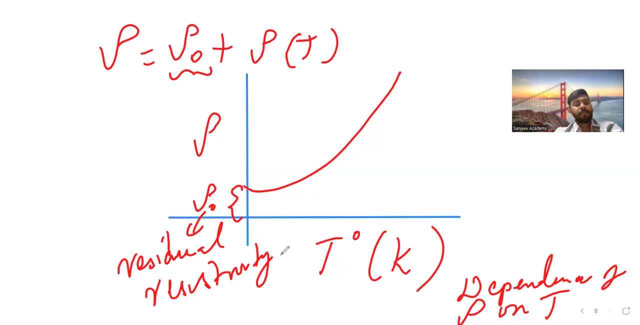 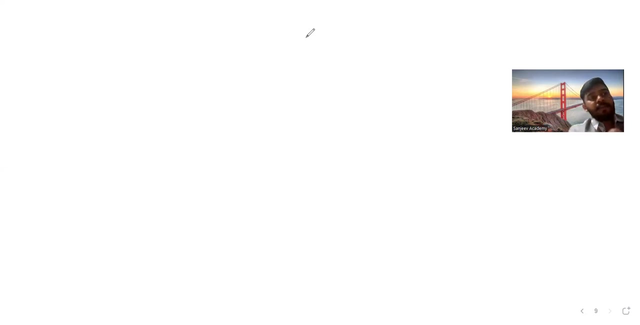 resistance left. so that is the limit, my raw, not now the most important thing in today's thing. i had to disapprove that cft is wrong, right, correct, cft is wrong. but before going to that, i'll just write down one more thing. this is my classical free electron theory. 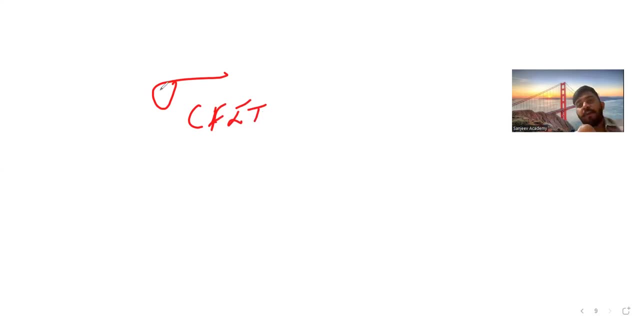 conductivity correct. the sigma is called conductivity. n e square tau by m. this again last year, class 12, current electricity chapter, we have learned n e square tau by m the derivation. okay, so coming to prove that this classical free electron theory is wrong, we have to check it on what we have done. so we have to check it on what we have done. 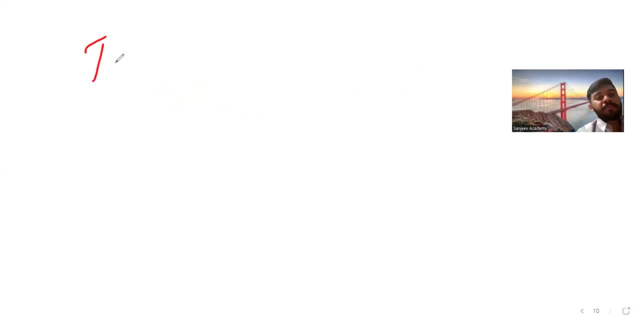 what? the temperature dependence on electrical conductivity. temperature dependence on electrical conductivity. okay, so experimental nature, correct sigma, this conductivity, experimental nature gave me what a? it is inversely proportional to temperature. it is inversely proportional to temperature, okay, but in the classifier, in the classic free electron theory. sigma, according to my classic.